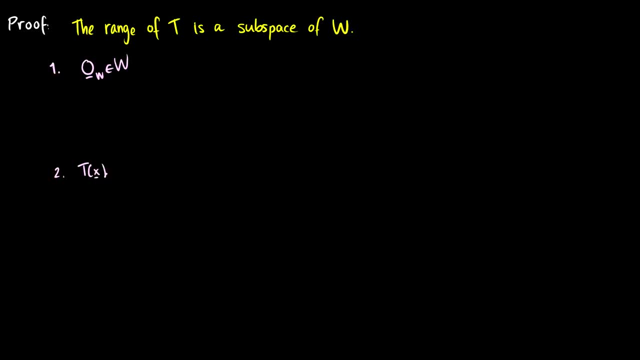 that if Tx and Ty are in W, then T of x plus y is in W. And then, of course, our third one: we have to check that if T times Cx is in W, this is the same thing as C times Tx. 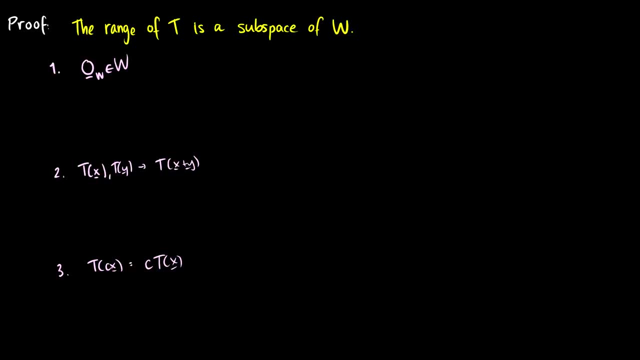 OK, so the first one. well, the nice thing about linear transformations is that we know that the transformation on the 0 vector in V is going to be the 0 vector in W. So this is a result of the definition. So, of course, if we take C times a vector, 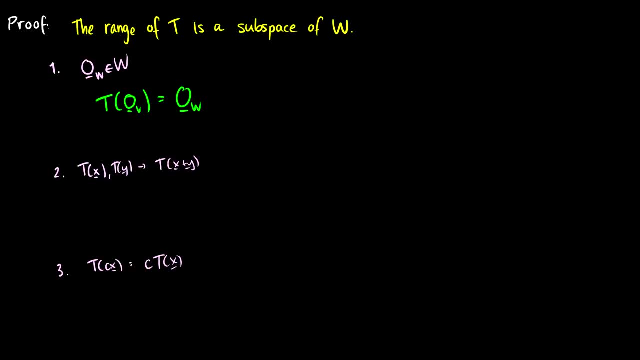 then we're going to get C times a transformation back. So if we put in 0 as our vector or we multiply it by 0, we're just going to get 0 back. So This one is from the definition of a linear transformation. 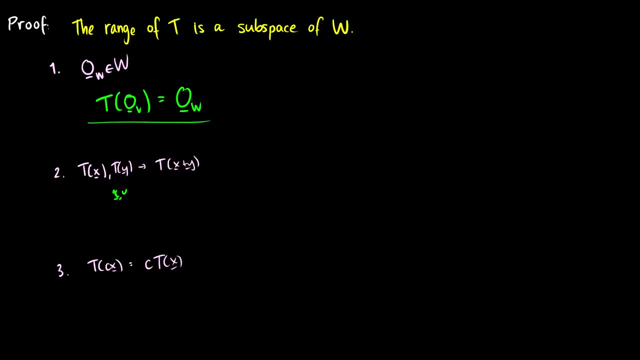 Two. OK, so we have to assume that x and y are going to be in V And this means that the transformations Tx and Ty are going to be in W. OK, well, with the definition, we know that the transformation of x plus the transformation 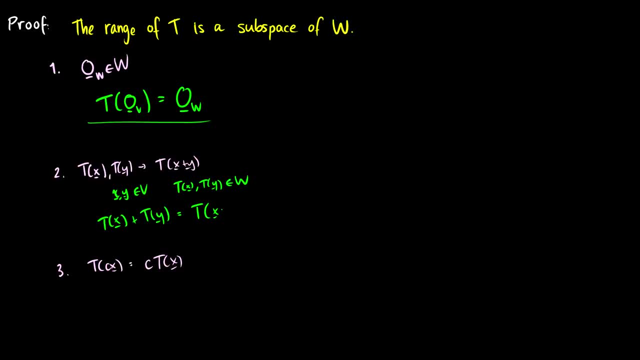 of y is going to equal the transformation of x plus y, And this is just the definition of a linear transformation. Therefore this one holds as well. OK, And of course, if we have an x in V and we have a C in the reals, then of course, 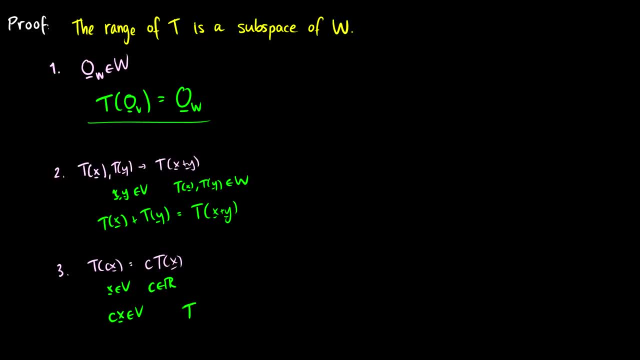 C times x is going to be in V, So we can take the transformation on C times x And we know this is going to be in W And T, or the transformation of Cx is the same thing as C. It's going to be in V times the transformation on x. 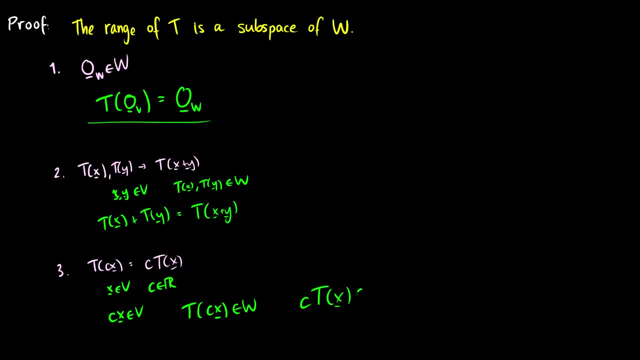 So that is also in the subspace. Therefore we've satisfied the three conditions. So we know that the range of T is a subspace of W. So these are all pretty much just by definitions. So this proof you should have been able to do on your own. 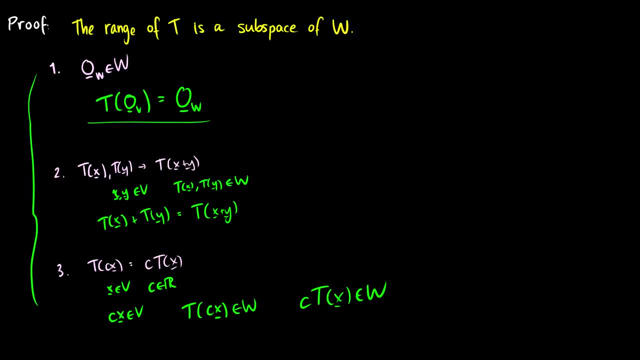 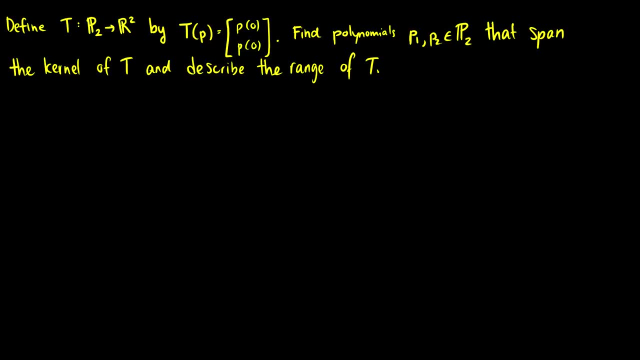 But for the sake of the video, that's how we go through that one. OK, This next question is going to be a little bit trickier, And I Was. It took me a little bit to do this the first time. 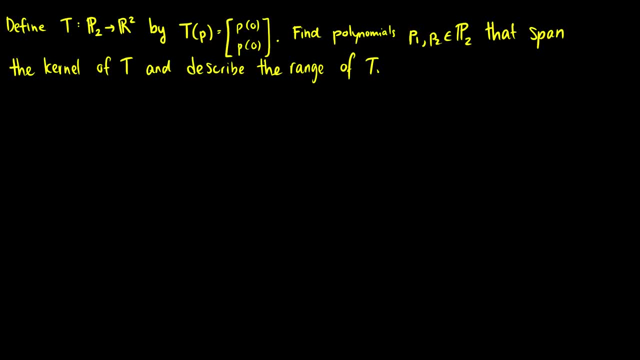 So just we're talking about R2, R3 all the time. We don't really talk about polynomials. So when you're thrown into this mindset of polynomials, things can seem a little bit tricky at first. Takes you a few seconds to wrap your mind around what. 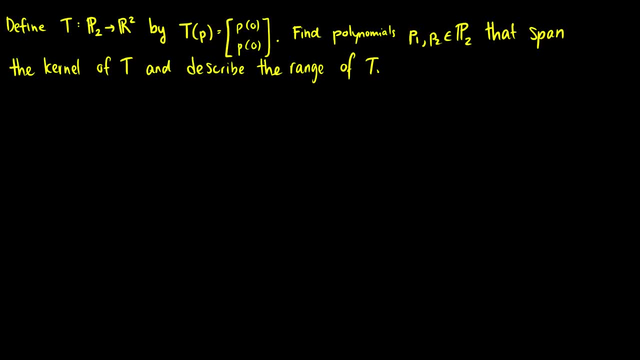 the question is asking and to solve it. So we have a transformation from P2 to R2.. So I'm going to draw this abstractly here, So I'm going to draw our spaces here, just so we can visualize what's going on. 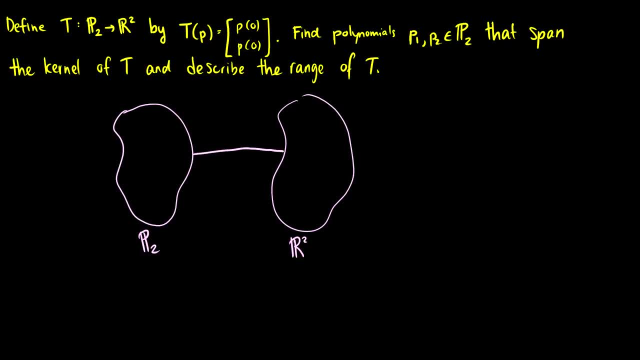 We have P2 to R2.. There's some mapping of T here And it maps the polynomial to a vector by evaluating the first entry of the polynomial at 0 and the second entry of the polynomial at 0. So we want to find two polynomials that. 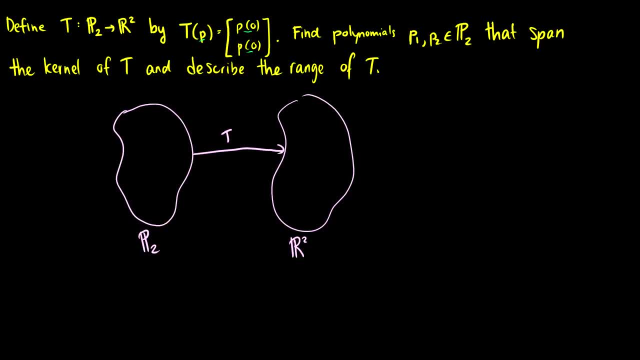 span the kernel of T, And then we want to describe the range of T. So, OK, Let's break this down. What is the question asking? So we want to find P1 and P2 that span the kernel of T. So we want to find two or one or two polynomials. specifically, 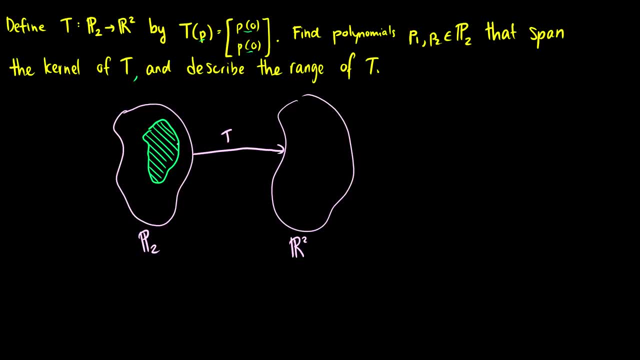 two polynomials here that will take any vector that maps to 0. And it describes the space. So we want R2 polynomials to 0.. And we want R2 polynomials to span this whole part on the left here. OK. 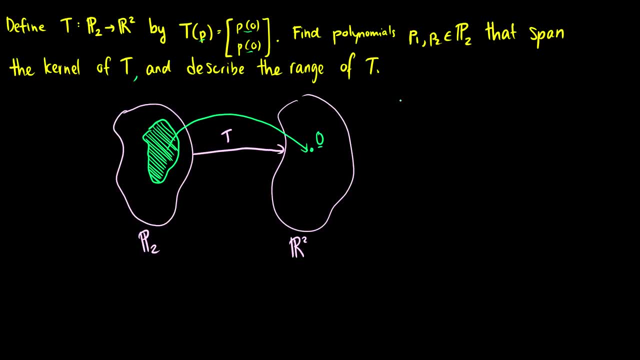 So what does a polynomial look like? first, Let's start with that. So a polynomial T is going to be a0 plus a1t plus a2t, squared. OK. So what is P0?? OK, We put in P0.. 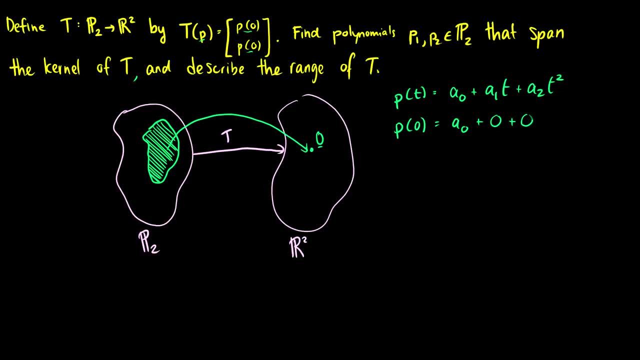 We put in a0 plus 0 plus 0, because we substitute 0 for Ts, And we're left with a0. So right away we can kind of see the range of this. So whatever we put in as our polynomial, 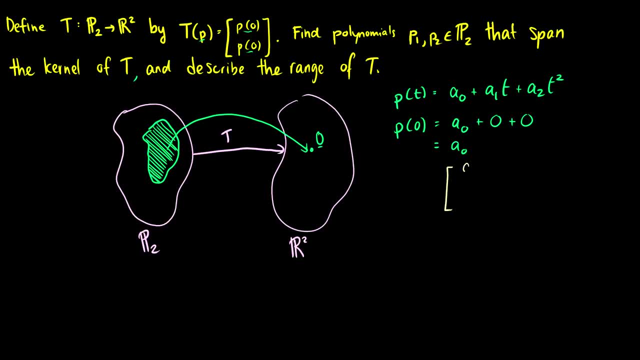 the transformation is going to take it to the matrix a0, a0.. And this will be for any a0 in the real numbers. So this is actually our range here. So Let's see, Write that down. That's the range. 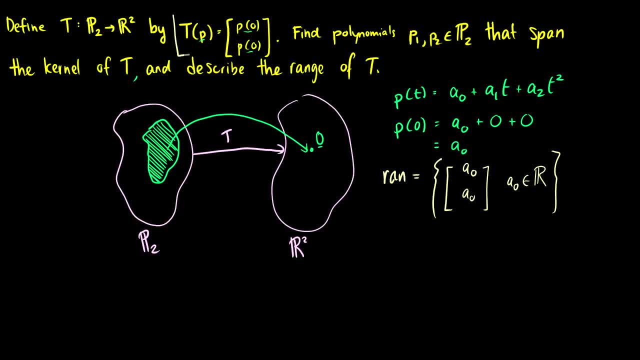 And, of course, this is just defined by the matrix given to us up here or the transformation given to us. OK, So now we'll find the polynomials that span the kernel of T. Well, these are all the things that go to 0.. 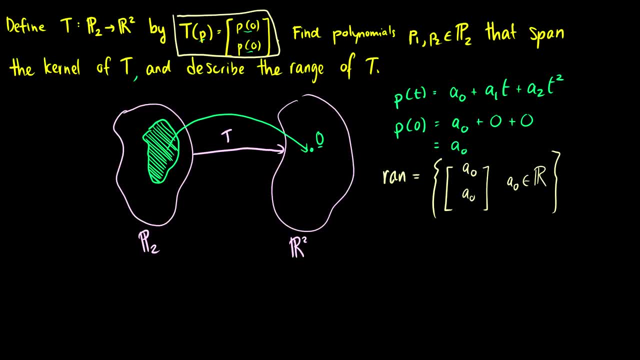 So let's assume that this a0 is equal to 0, because then we'll get the 0 vector. So we're going to take Pt And a0 is going to equal 0, because that way we'll get 0.. 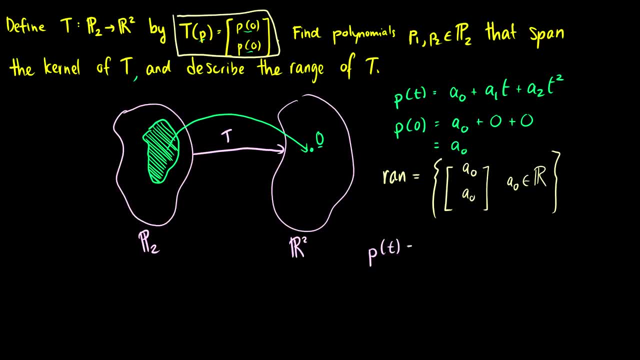 0, 0 out of there, And we're just going to be left with a1t plus a2t squared. OK. Well, I can kind of see two polynomials here, So we want two polynomials that span the kernel of T. 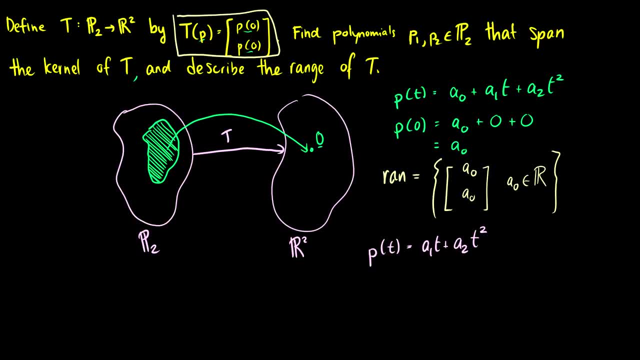 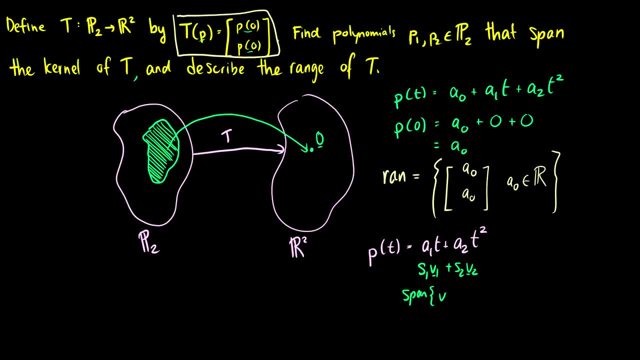 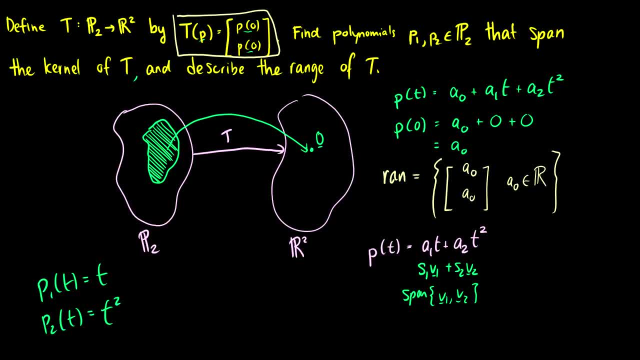 And our second polynomial, T, is just going to be T squared. And that is because, if we take a look at this, we can see this is a linear combination. So we can match up these linear combinations And then we can relate it to the span. 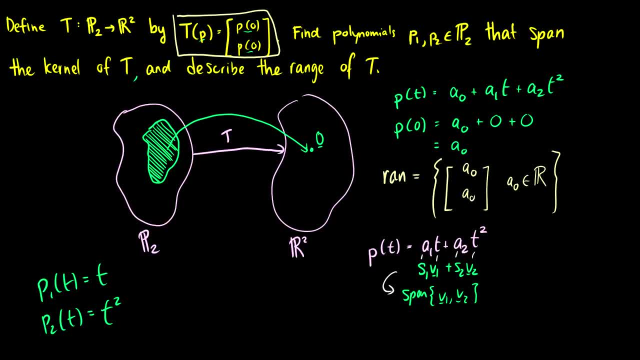 So working in polynomials a little bit different than working in the plane. So r2, r3, you need to get a different mindset. You have to remember the definition of the polynomial, which is definitely the hardest part to remember because you're not going.